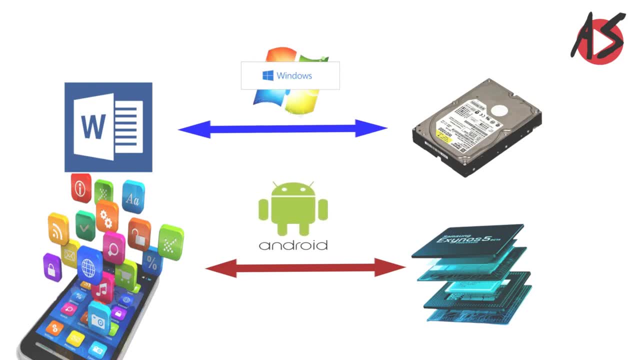 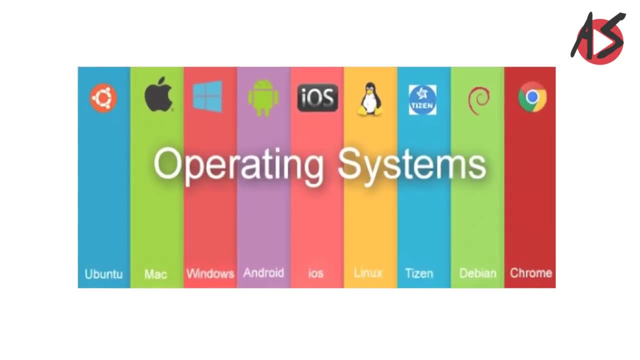 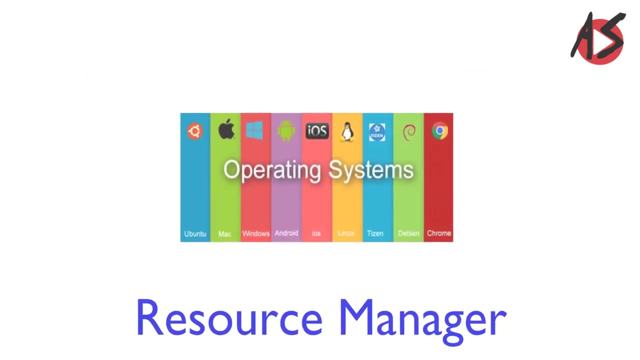 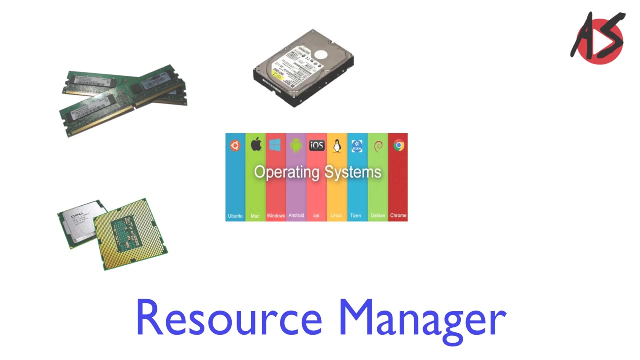 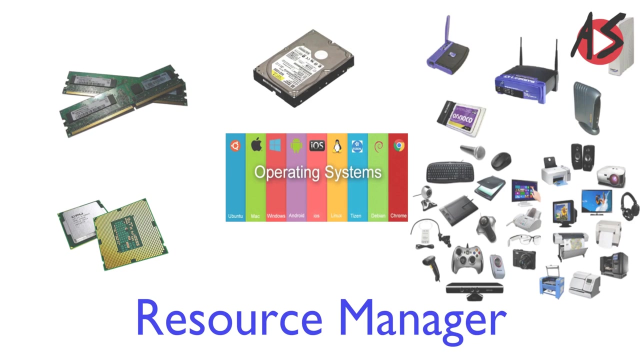 Or we can say it will interact with the hardware. That is called operating system or OS. Operating system is also called resource manager, Which manages all the resources, That is, hardware, including CPU, RAM, Disk, Network and Input Output devices. Popular operating systems are Windows, Linux, Android and Macintosh. 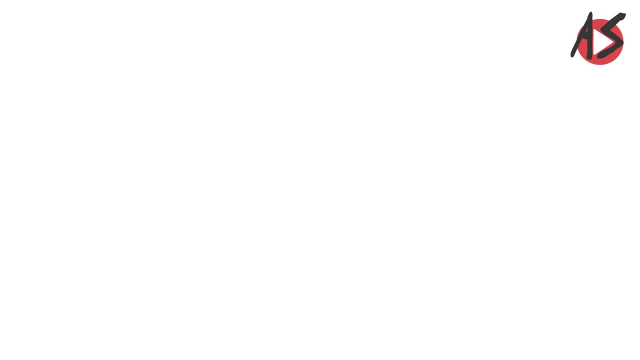 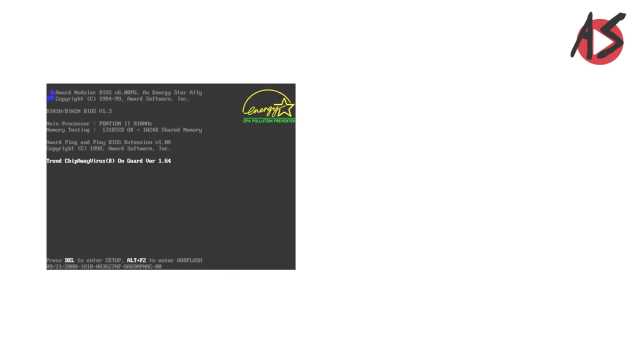 When the computer is turned on, it first performs the power on self-test, And if no issues are found, the bootstrap loader will load the operating system for the computer into memory. Now you know what is a bootstrap loader. Now you know what is a bootstrap loader. 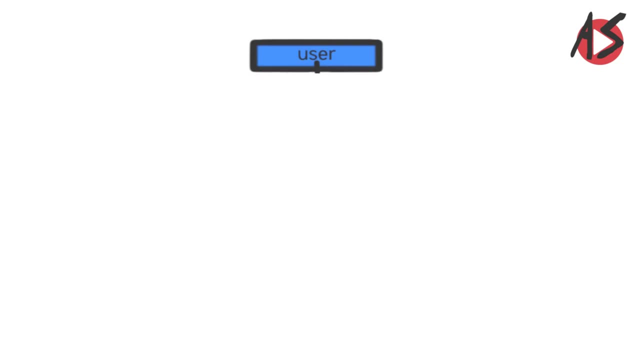 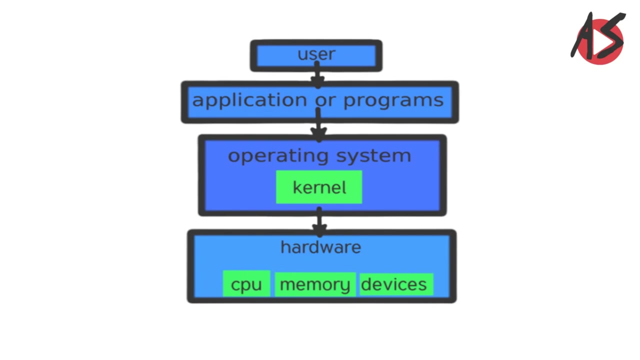 Now you know what is a bootstrap loader. Now user can start interact with the computer via applications and program. This application program internally use operating system, Operating system core part which is called kernel. interact with the hardware like CPU memory and all kind of input output devices. 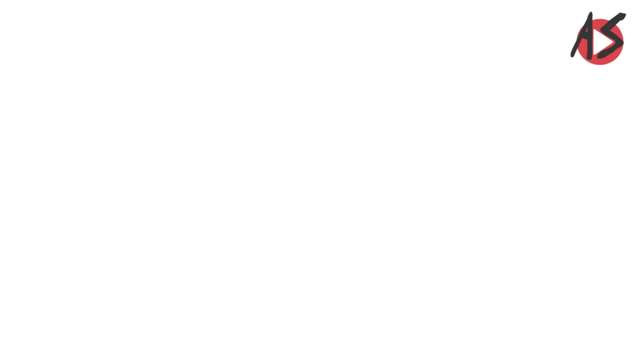 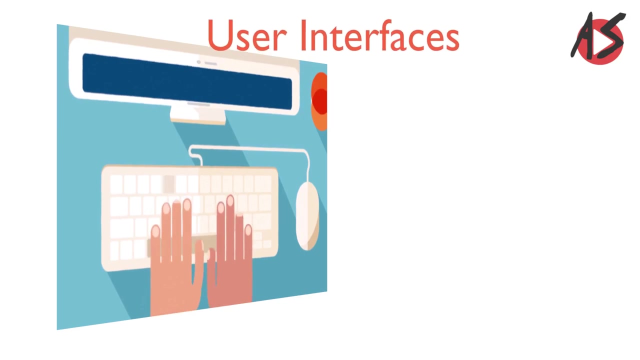 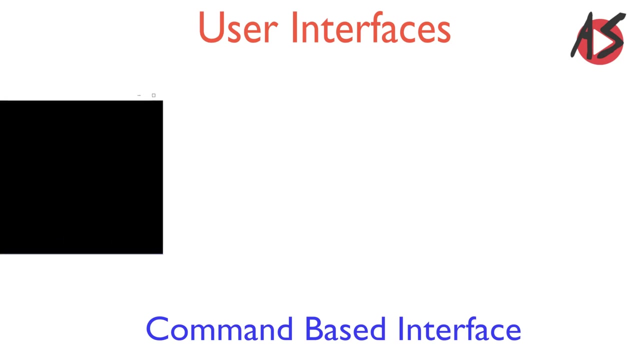 The objective of an operating system. Operating System is to provide an interface to the user through which the user can interact with the computer. There are many types of user interfaces. Let's see one by one. Command-Based Interface: Command-Based Interface requires a user to enter the command. 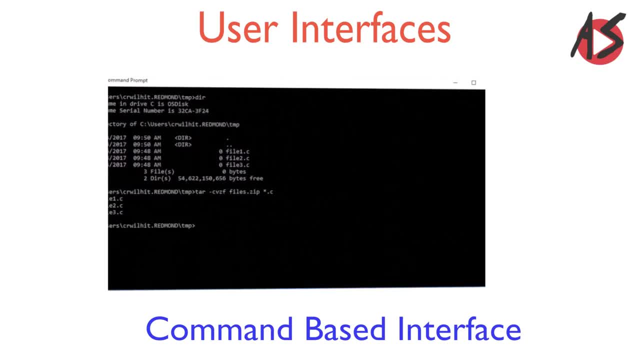 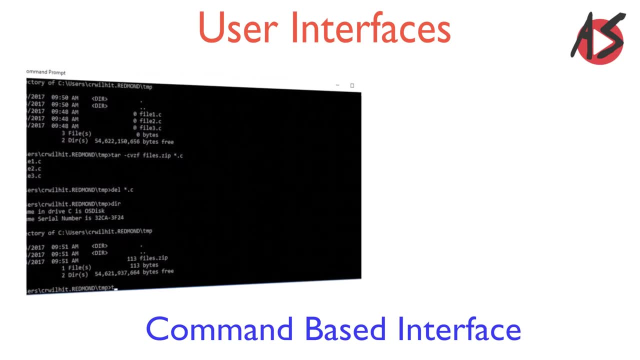 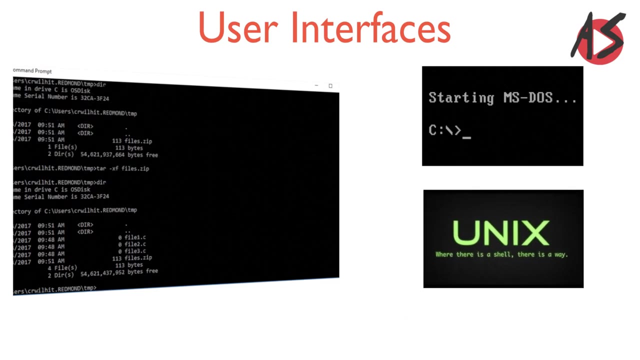 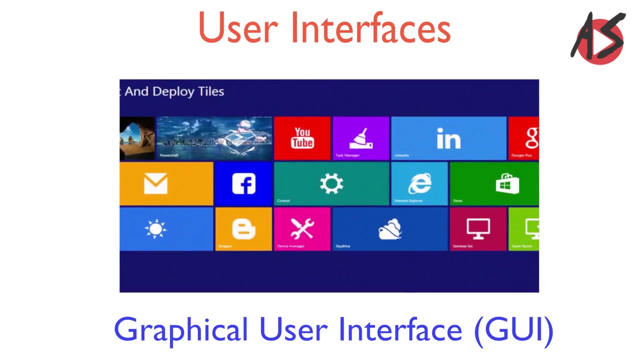 to perform different tasks like creating, opening, editing or deleting a file. Examples of Operating Systems which Command-Based Interface include MS-DOS and Unix. Graphical User Interface- Graphical User Interface, also known as GUI, lets user run program or interface. 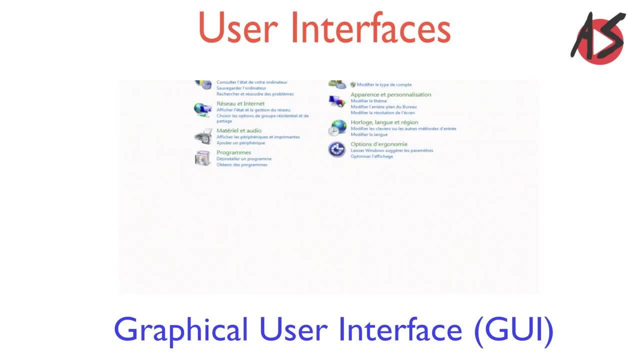 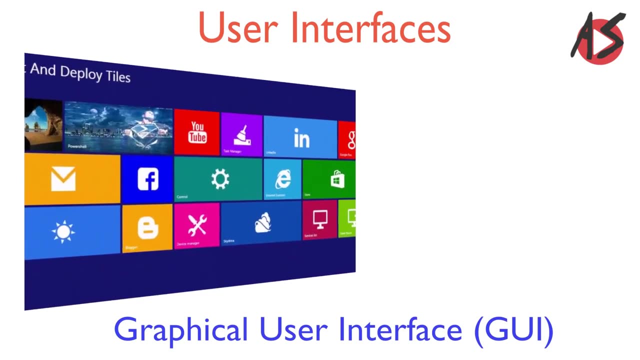 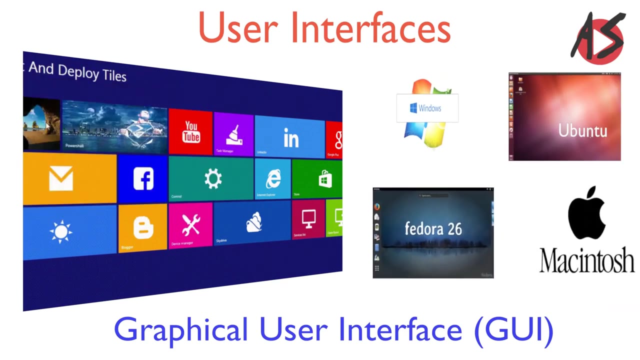 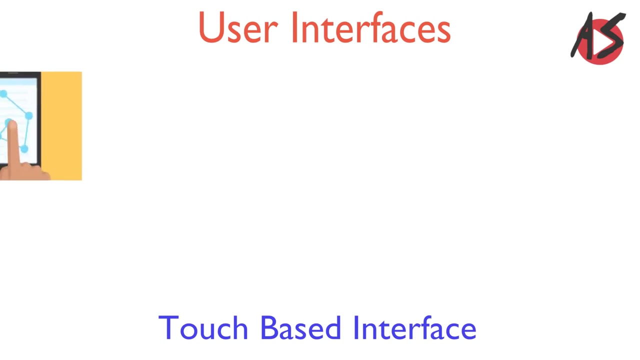 Command-Based Interface can interact with computers in the form of icons, menu and other visual options. Examples of GUI-Based OS are Microsoft Windows, Ubuntu, Fedora and Macintosh Touch-Based Interface. Today's smartphones, tablets and PCs allow users to interact with. 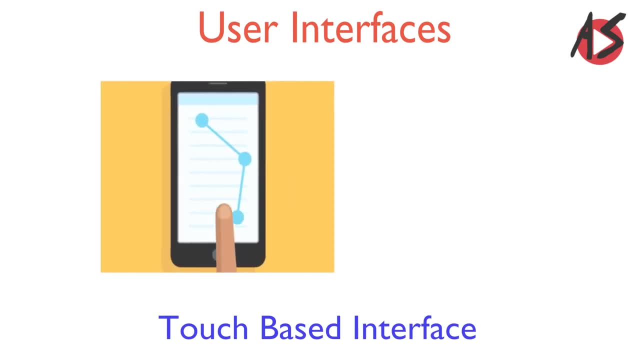 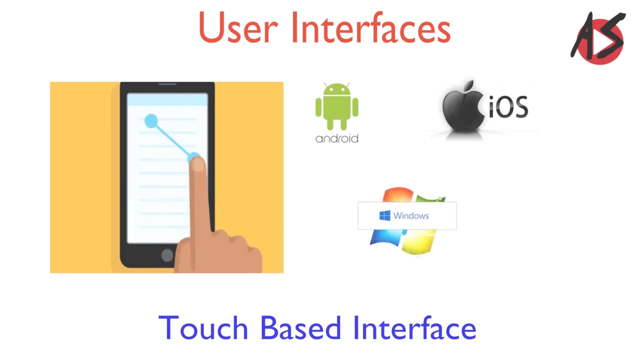 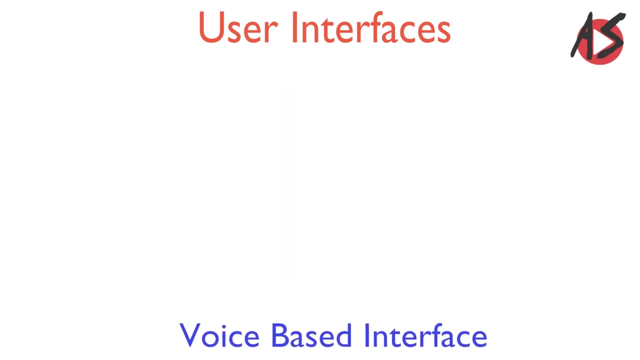 the system simply using the finger-touch. Examples of Popular Operating Systems which Touch-Based Interfaces are Android and iOS. Modern Window Operating System is also support Touch-Based Interfaces on touchscreen devices. Voice-Based Interface: User today can use voice-based command-based interface to interact with the system. 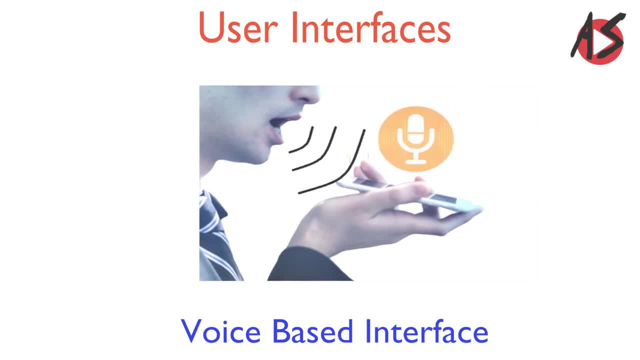 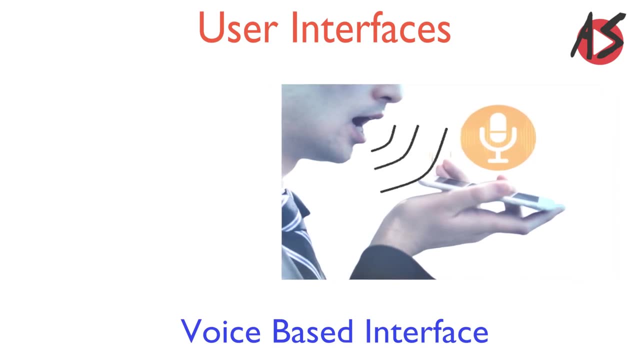 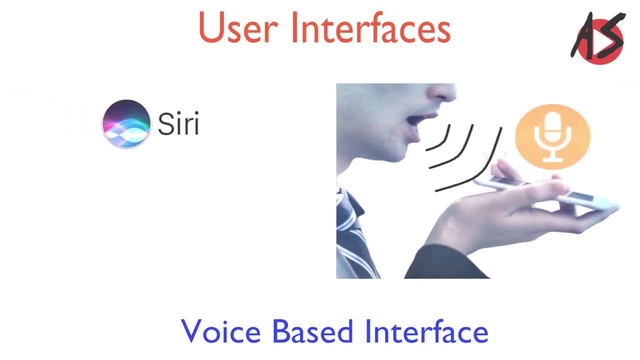 Command-Based Interface. User today can use voice-based command-based interface to interact with the system. Functional Interface can interact with the system by swaqu your mouse on the VM ID. Tucker Connector cannot be used. Buffalooseą' the next-generation gentlemen. General Software-based13EST 들어�. navy Can drive a computer to the web with multiple smart media applications by built-in Bluetooth rack between options to 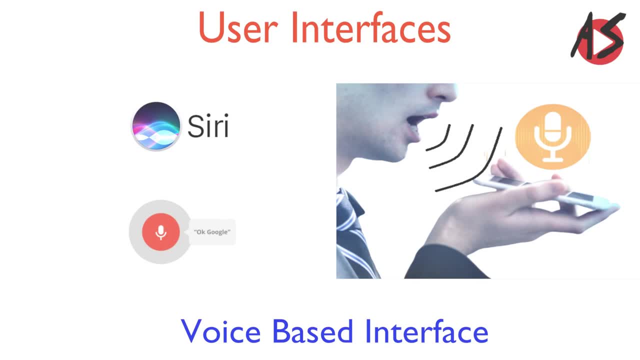 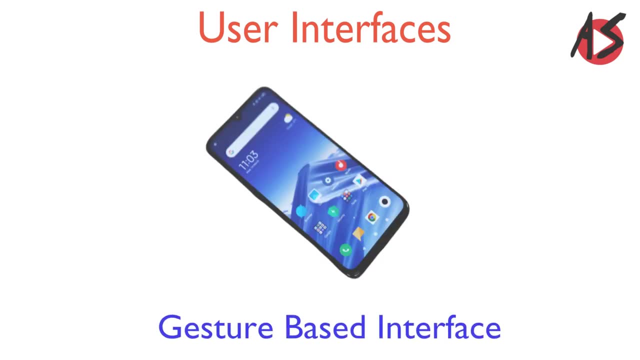 wordten and make a computer work in a desired way and give the input without keyboard or mouse or touch screen are few examples of voice-based interfaces. gesture-based interfaces, Some smartphones based on Android and iOS, as well as laptops, let users interact with the device using gestures like waving, tilting and eye motion. 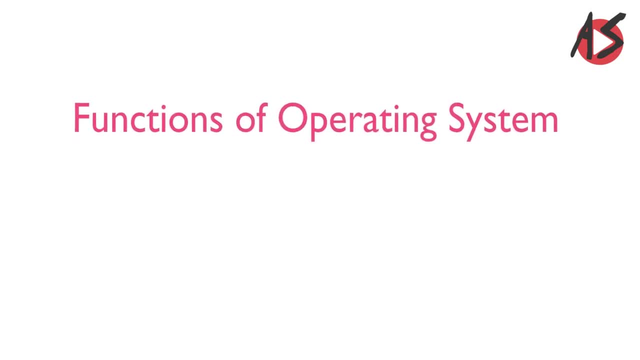 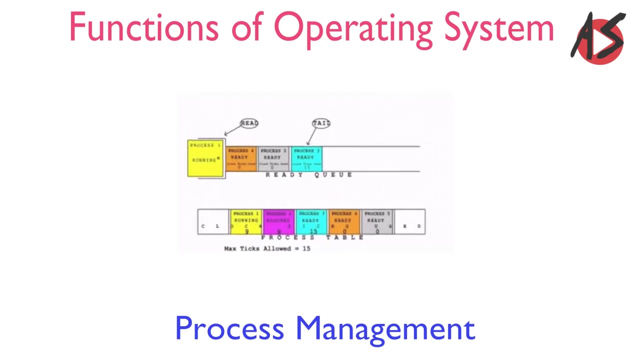 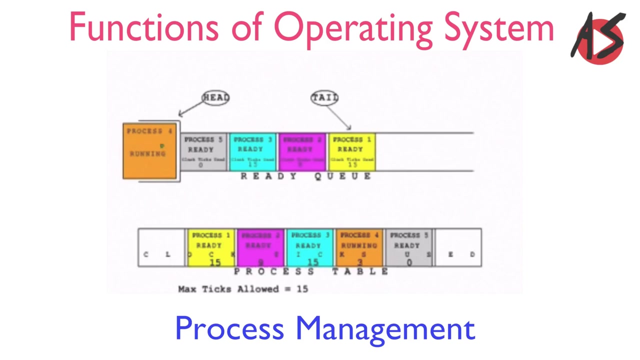 Now we will see important functions of operating system PROCESS MANAGEMENT. In computer, different processes are running simultaneously. It is the responsibility of operating system to manage these processes and get multiple tasks completed in minimum time. As CPU is the main resource of the computer system, Its